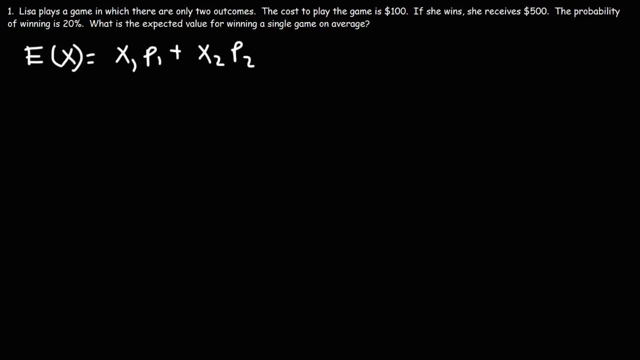 So let's begin by organizing the data in this problem in the form of a table. So first we're going to write the outcomes. There's really only two outcomes that we need to be concerned with: Either she wins the game or she loses. 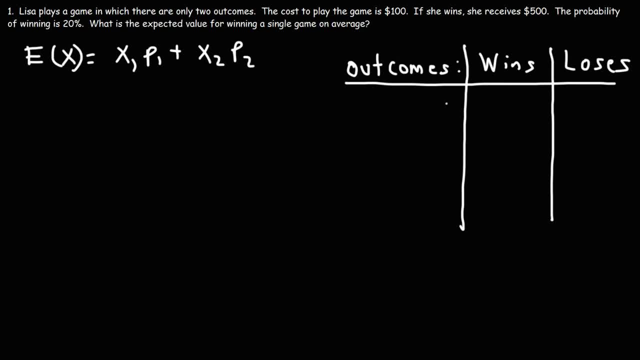 Now, the next thing we need to concern ourselves with is the value of each outcome. If she wins the game, she receives $500.. If she loses the game, well, the cost of play is $100, so she's going to lose $100. 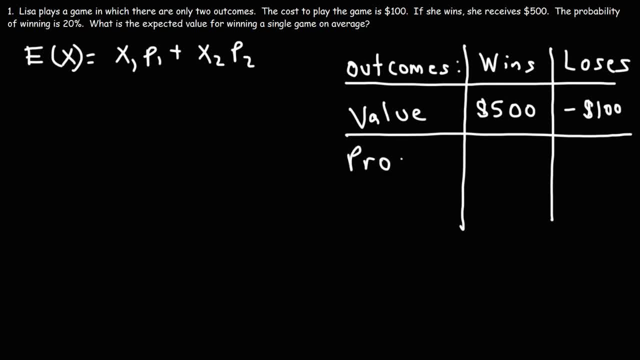 The next thing is the probability of each outcome. The probability of each outcome is the value of each outcome. The probability of each outcome is the value of each outcome. The probability of Lisa winning the game is 20%, according to the problem. Based on that, what is the probability that she's going to lose? 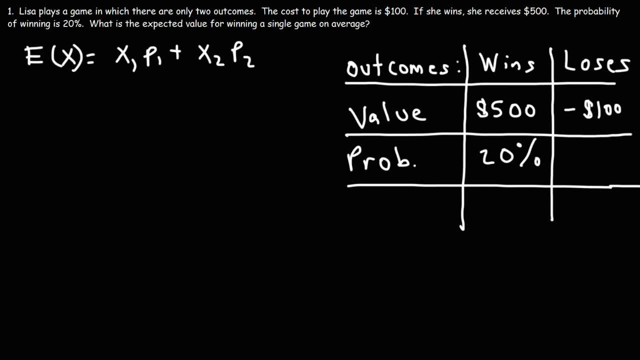 Well, we know that the maximum probability is 100%, So there's a 20% chance that she's going to win the game. There's an 80% chance that she will lose the game, since there's only two outcomes. So now we have enough information to calculate the expected value for winning this game. 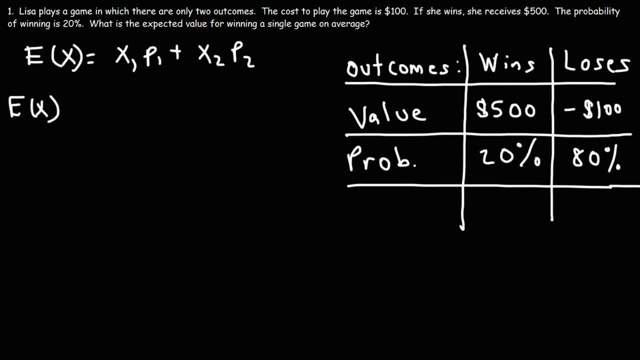 So this is going to be number 1, and this is number 2.. So x1 is the value of winning the game. That's going to be $500.. P1 is the probability of winning, So we need to convert the percentage into a decimal. 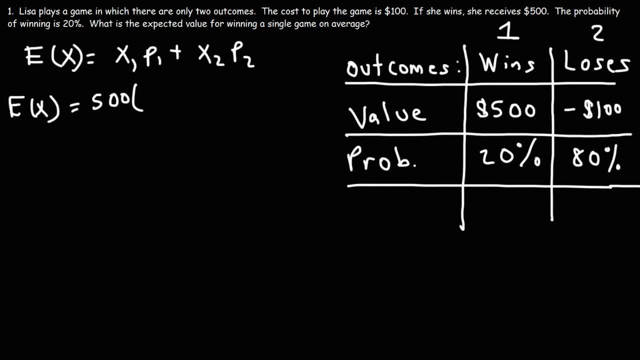 To convert percent to a decimal divide by 100, or you can move the decimal point two units to the left. So 20% as a decimal is .20.. Now x2 is the value of losing the game. In this case, that is negative 100.. 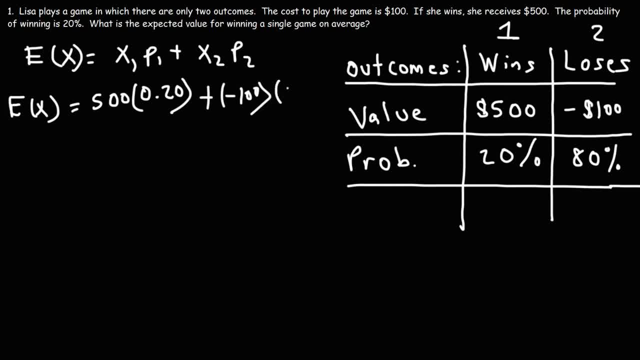 P2 is the probability of losing, which is 80% or .80.. Now, 500 times .20, that is 100.. And negative 100 times .80 is negative 80. So the expected value of losing the game is .80.. 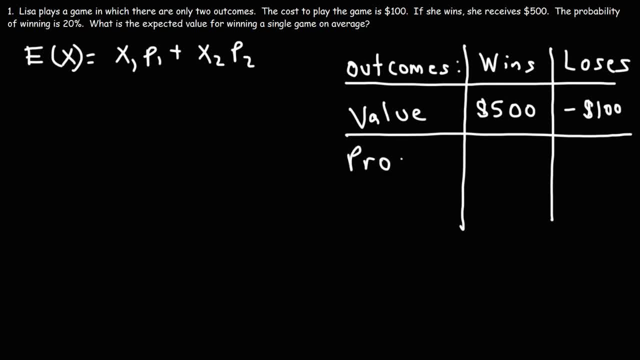 The next thing is the probability of each outcome. The probability of each outcome is the value of each outcome. The probability of each outcome is the value of each outcome. The probability of Lisa winning the game is 20%, according to the problem. Based on that, what is the probability that she's going to lose? 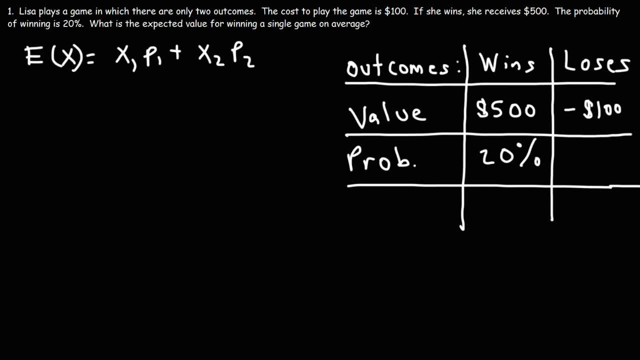 Well, we know that the maximum probability is 100%, So there's a 20% chance that she's going to win the game. There's an 80% chance that she will lose the game, since there's only two outcomes. So now we have enough information to calculate the expected value for winning this game. 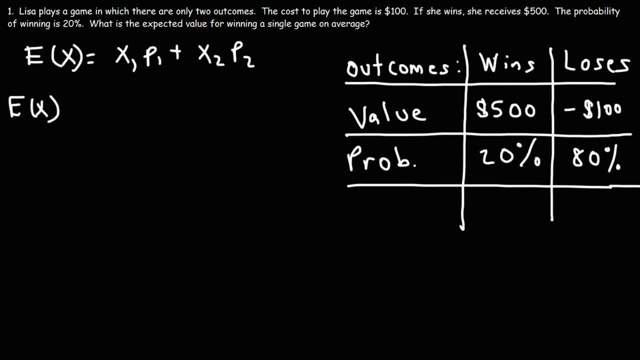 So this is going to be number 1, and this is number 2.. So x1 is the value of winning the game. That's going to be $500.. P1 is the probability of winning, So we need to convert the percentage into a decimal. 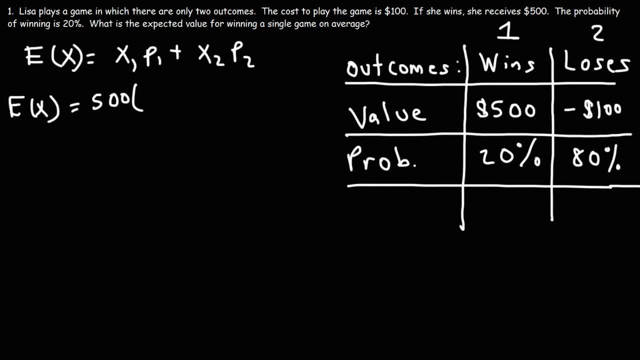 To convert percent to a decimal divide by 100, or you can move the decimal point two units to the left. So 20% as a decimal is .20.. Now x2 is the value of losing the game. In this case, that is negative 100.. 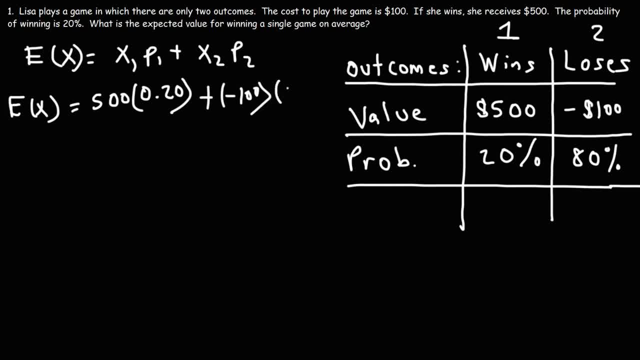 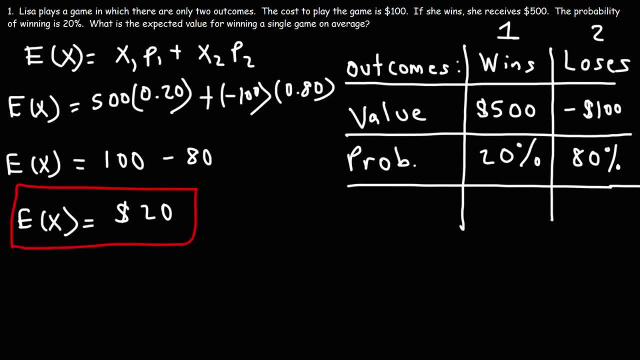 So the expected value of losing the game is .80.. on average, if she continues to play this game, she can earn $20 per game. Now how much would she expect to win? let's say, if she were to play 10 games? 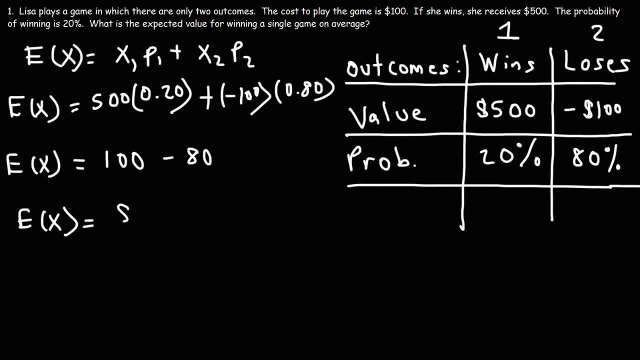 So the expected value of losing the game is .80.. So the expected value of winning a game on average is 10 where. So on average, if she continues to play this game, she can earn $20 per game. Now how much will she expect to win? 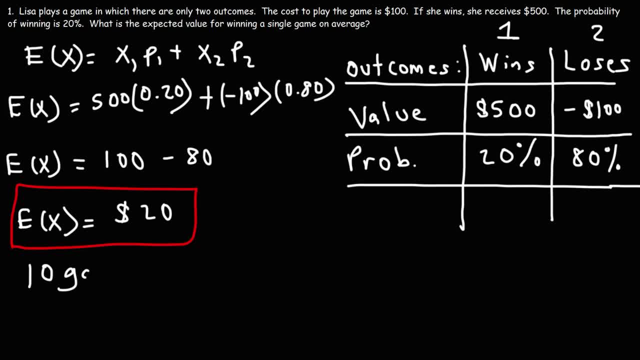 let's say, if she were to play 10 games, Well, if she can average $20 per game, then 10 games would would at this rate case, if she continues to play this game, 10 games per 45 minutes. 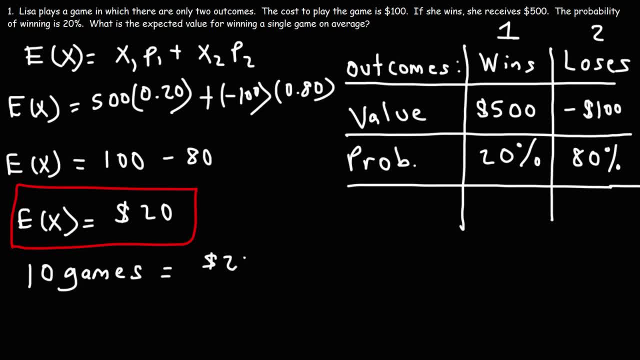 rate. give her an expected earnings of $200. if she were to play a hundred games. based on this average earnings, she would expect to have a total of 2,000 at that point, and so that's how you can calculate expected value for winning a single game, and then you could use that to estimate what your total earnings. 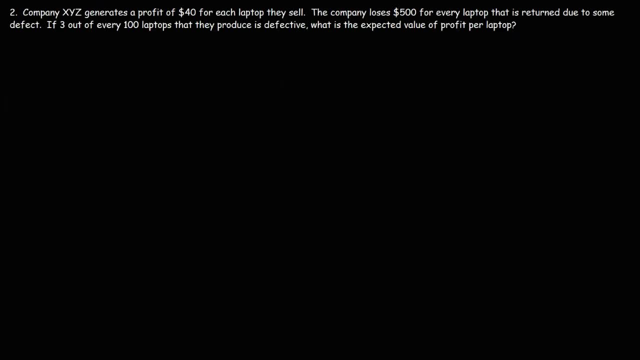 will be for playing a certain number of games. now let's work on another example problem. company XYZ generates a profit of $40 for each laptop that they sell. the company loses $500 for every laptop that is returned due to some defect. if three out of every laptops. or, let me say that again, if three out of every 100. 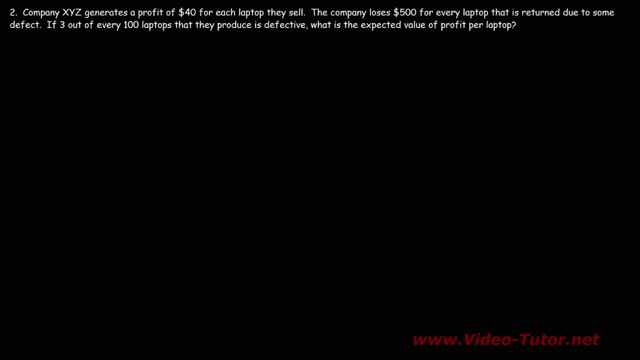 laptops that they produce is defective. what is the expected value of profit per laptop? well, let's write down what we know you. so in this problem, similar to the last one, there's only two outcomes that we need to be concerned with: either the company makes a working laptop or defective. 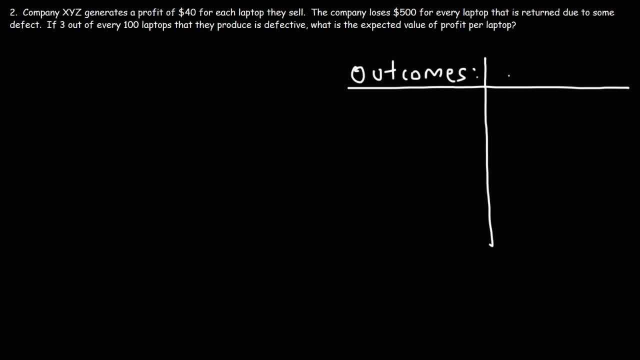 one. so let's say, if they generate a working laptop, that's a win for them, and if they make a defective laptop, that's basically a loss for them. so the value of making a laptop that is functioning properly is $40. that's how much they're. 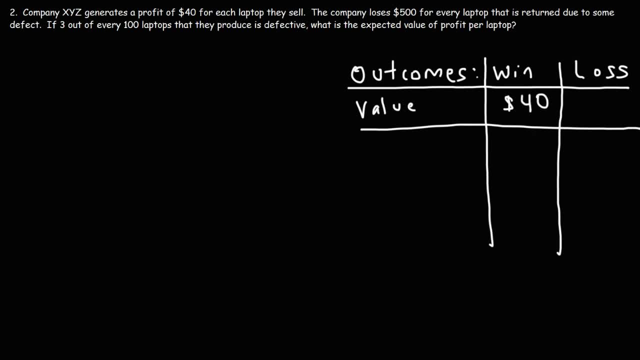 gonna profit for each properly working laptop that they sell. now. if they make a defective laptop, they're gonna lose $500. so that's a huge loss. it takes a lot of money to make a laptop. and now the probability of making a working laptop? well, let's find the probability of making a 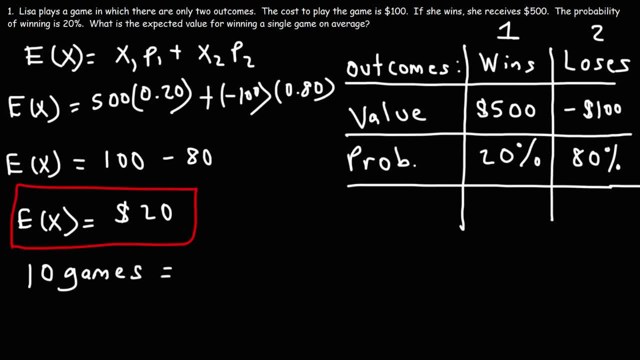 Well, if she can average $20 per game, then 10 games would, at this rate, give her an expected earnings of $200.. If she were to play 100 games, based on this average earnings, she would expect to have a total of $2,000 at that point. 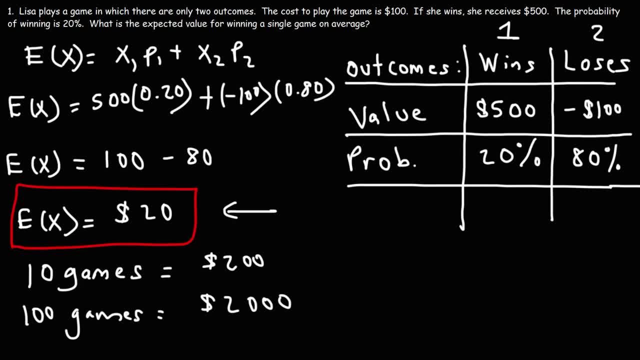 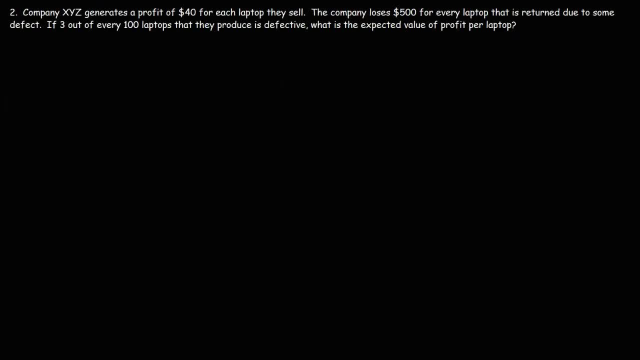 And so that's how you can calculate expected value for winning a single game, and then you could use that to estimate what your total earnings will be for playing a certain number of games. Now let's work on another example problem: Company XYZ joined the game. Now let's work on another example problem: Company XYZ joined the game. 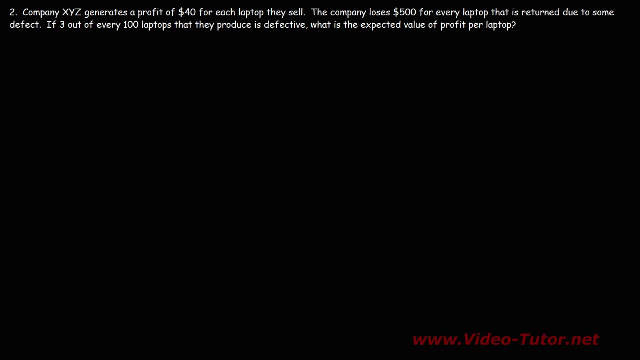 Now let's work on another example problem. Company XYZ joined the game. This company generates a profit of $40 for each laptop that they sell. The company loses $500 for every laptop that is returned due to some defect. If three out of every 100 laptops that 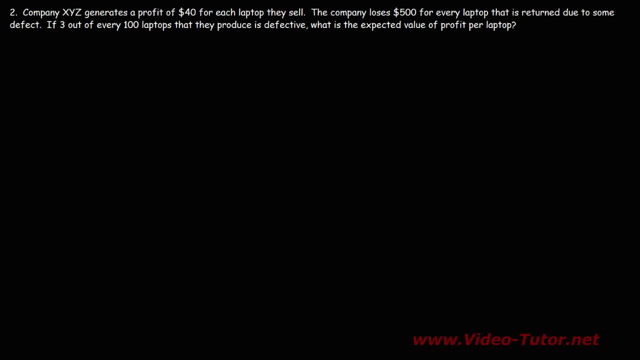 they produce is defective, what is the expected value of profit per laptop? Well, let's write down what we know. So in this problem, similar to the last one, there's only two outcomes that we need to be concerned with: Either the company makes a working laptop or a defective one. So let's say, if they generate 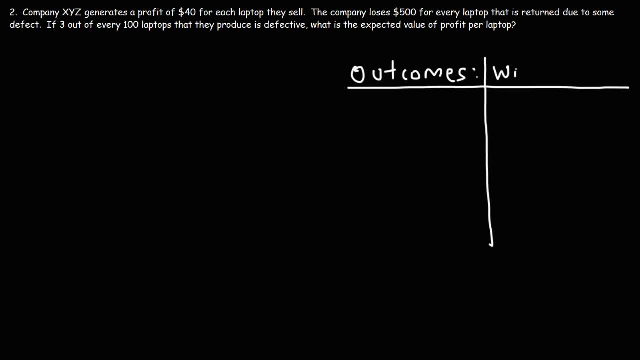 a working laptop, that's a win for them, And if they make a defective laptop, that's basically a loss for them. So the value of making a laptop that is functional is the same as the value of a laptop that is functioning properly. That's $40.. That's how much they're going to profit for each. 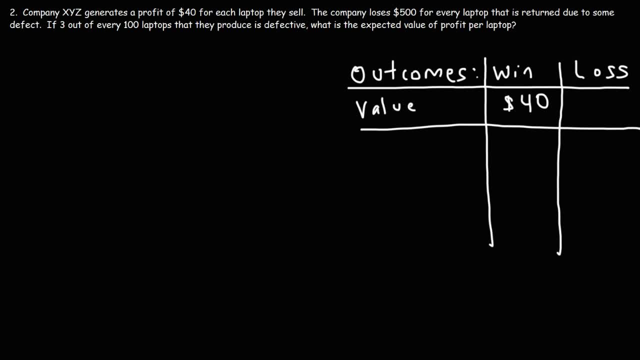 properly working laptop that they sell. Now, if they make a defective laptop, they're going to lose $500. So that's a huge loss. It takes a lot of money to make a laptop. And now the probability of making a working laptop. well, let's find the probability of making a defective laptop, Three out of every.